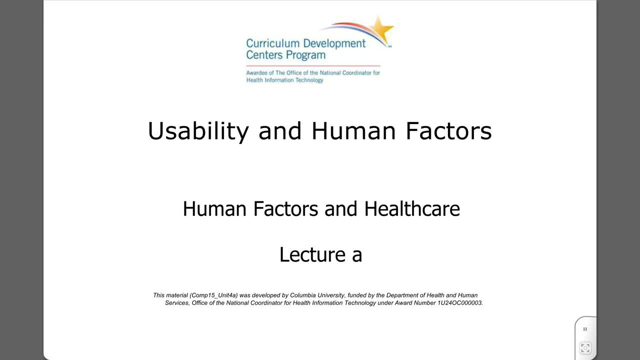 issues and concepts, as well as an introduction to the analysis of human error. The focus is on understanding the nature of human error and appreciating a system-centered approach which emphasizes the multiplicity and complexity of causes of human error. We then turn our attention. 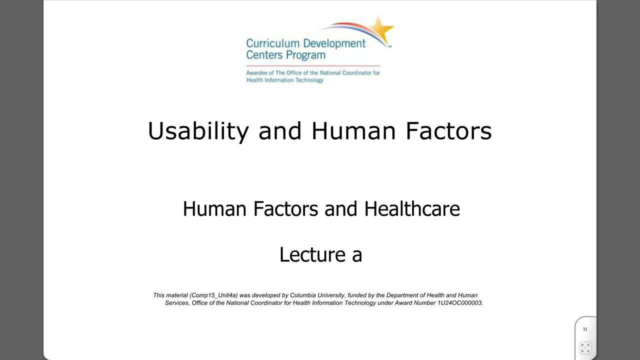 to workload, which is an important construct pertaining to the potential for error in a work setting. In the final section of this unit, we will examine medical devices and discuss two human factor studies that examine efficacy of such devices in clinical and home health contexts. 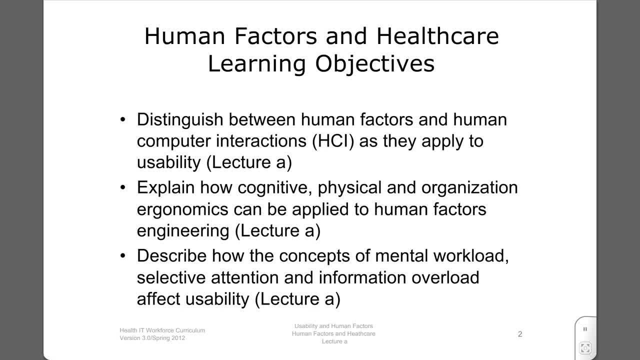 This unit covers the following objectives: 1. Distinguish between human factors and human computer interactions, HCI as they apply to usability. 2. Explain how cognitive, physical and organization ergonomics can be applied to human factors, engineering. and 3. Discretion. 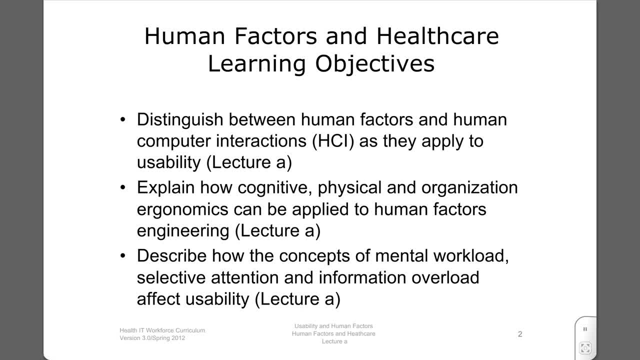 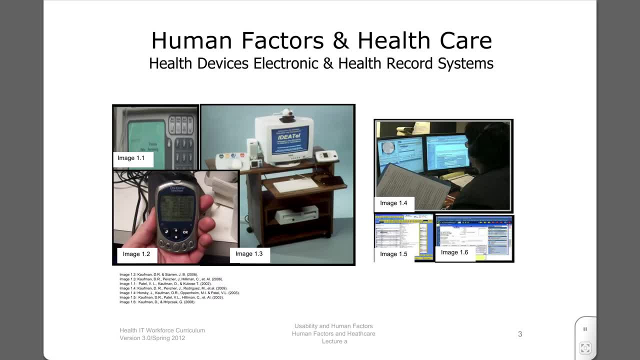 4. Describe how the concepts of mental workload, selective attention and information overload affect usability. Human factors is a discipline devoted to the study of technology systems and how people work with them or are affected by them. It is concerned with the full range of health. two Popeye. 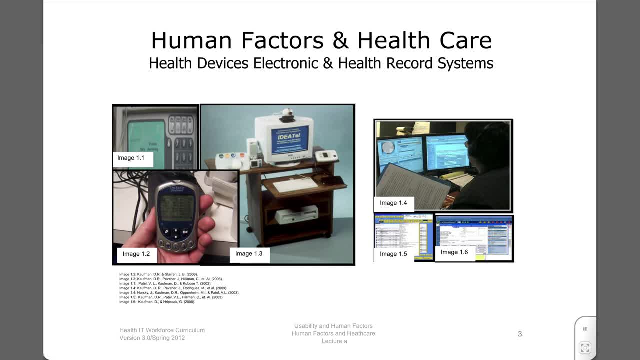 related technologies and systems used by a diverse range of people, including cliniciansts, üç Hospital administrators, ioань hailth, consumers and patients. and patients is a discipline that that Nephite, or the US national federal health, 是 to the United States. specifically, It has the capability of two. whoever work in a 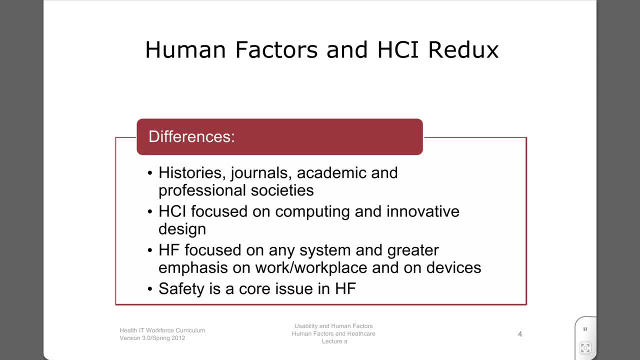 In this course we will frequently talk about both human factors and human-computer interaction, HCI. They are different disciplines with different histories and different professional and academic societies. HCI is more focused on computing and cutting-edge design and technology. Human factors- HF- focus on a range of systems that covers a wider range of hospital and other 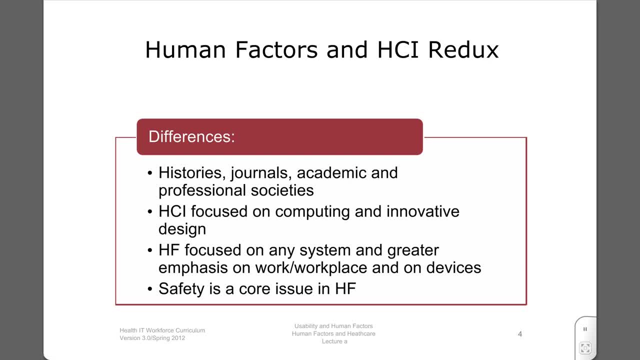 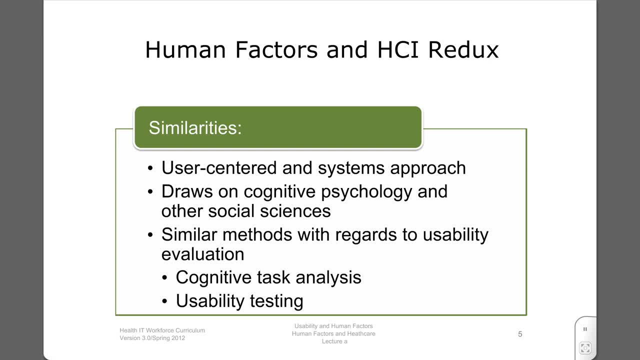 technologies. Patient safety is one of the central issues in human factors research. However, the two domains employ many of the same methods of evaluation and both strongly emphasize a user-centered approach to design and a system-centered approach to the study of technology use. Researchers and professionals in both domains draw on the same set of theories. 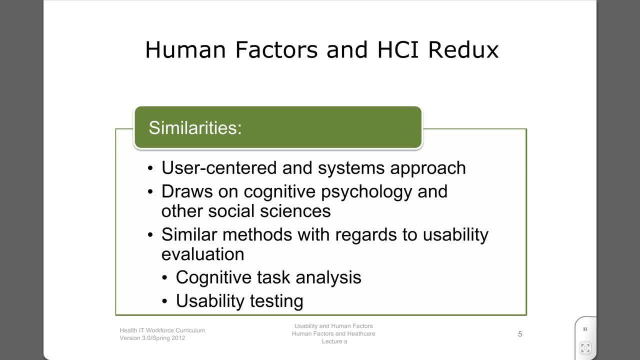 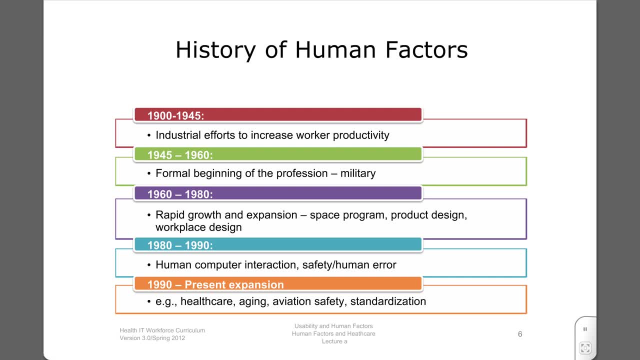 including cognitive engineering. This slide covers the history of human factors from the earliest efforts of engineers to increase the productivity of factory workers by changing environmental conditions. The discipline became formalized towards the end of World War II and shortly thereafter began an age of great expansion. 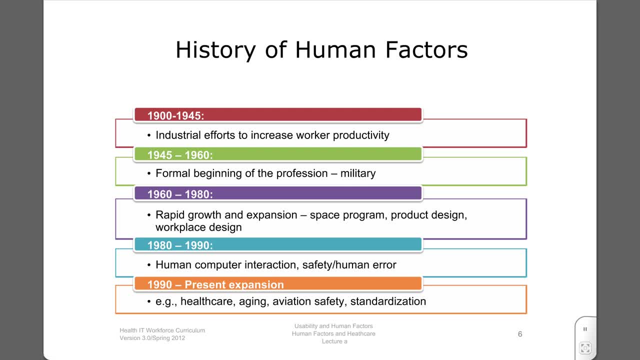 This time corresponded to the beginning of the space age and the rapid growth of the automobile industry, as well as aviation. The last 20 to 30 years have witnessed a considerable growth of the discipline in scope and importance. Healthcare has also become a focal 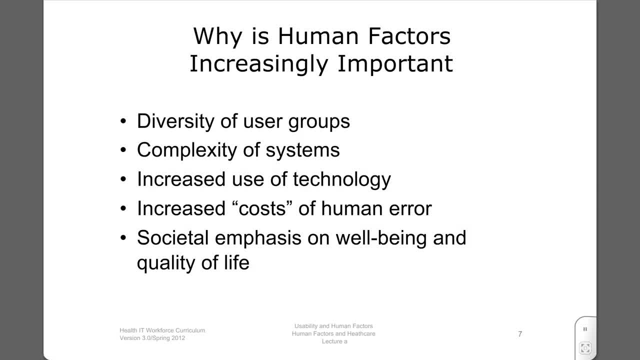 point of work in human factors. Human factors have grown in importance and in public awareness in recent decades. Some of this is due to an increase in the use of technology by diverse population of users, most of whom are not experts, a growing awareness of safety and the cost of error In 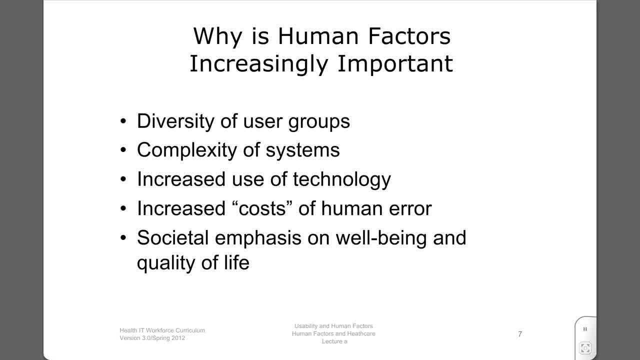 industry. there is an increasing recognition of the need for better service and better care, for the better quality control and the fact that it conveys a competitive edge. The car industry is a case point. There is a general perception that Japanese and European cars are of greater quality, and this 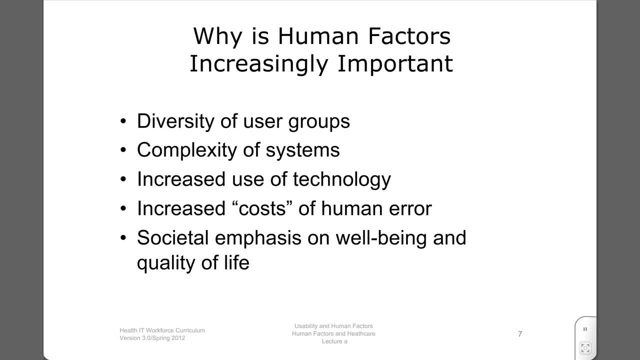 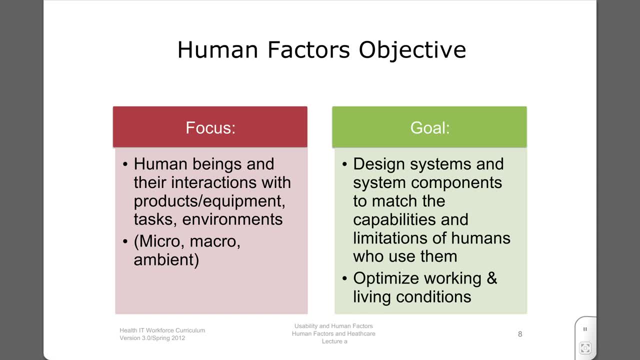 has hurt the sales of North American cars. What is the central focus of HF work? Broadly, it is humans and their interaction with the gamut of technologies and systems. The goal of this work is to optimize these technologies such that they match the capabilities and limitations of humans who use them As we. 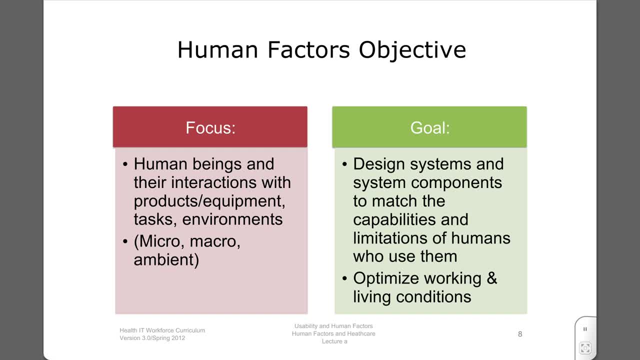 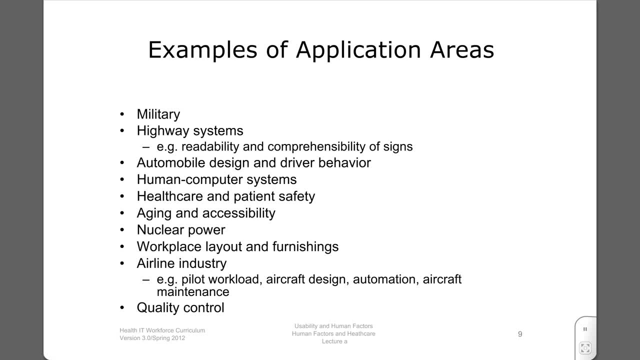 will discuss. cognitive psychology plays a very important role in human factors analysis. These are just some examples of application areas and human factors. We will focus on computer systems and patient safety, but we will also touch on other areas. Here is a picture of a control room. 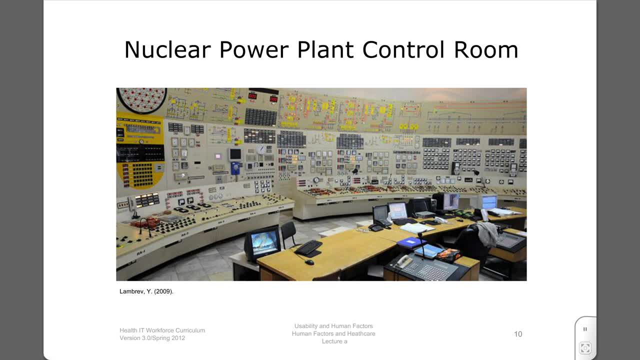 plant Safety is a crucial issue in these settings. Homer Simpson is probably not the embodiment of the ideal nuclear power safety inspector, although he is the best known. The picture illustrates the immense complexity of such an environment, and one can imagine the demands on human operators. 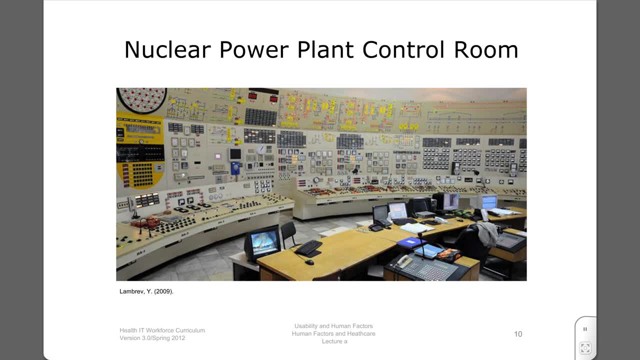 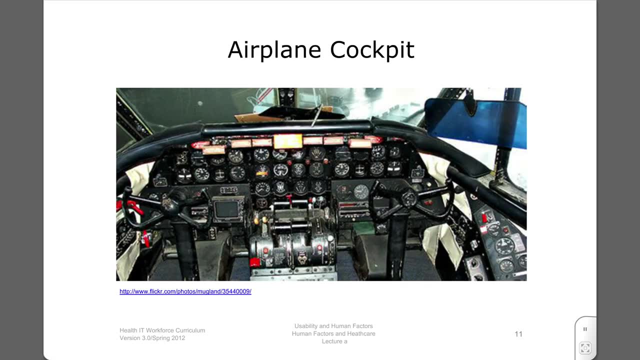 There have been several significant accidents in such plants, and they have served as excellent case studies in human factors engineering. The aviation industry is one of the first to embrace the discipline of human factors as well as human factors engineering principles, Although airplane crashes make the front pages of our newspapers when they happen. 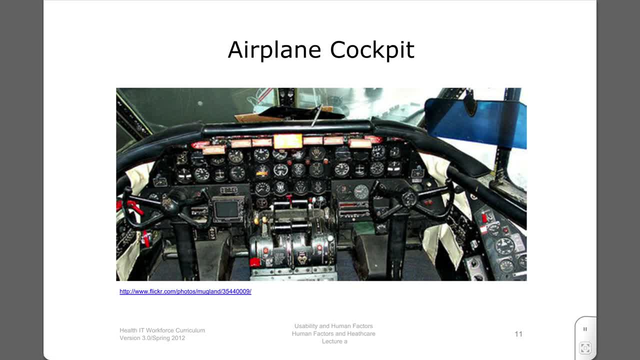 the airline industry has an excellent safety record. in recent decades They have evolved a rather elaborate set of procedures for ensuring safe practices, which includes rigorous training of pilots and ensuring maintenance of pilots' competencies. We hear about the failures in aviation, but on balance they set a high standard on matters of safety In the last decade or so. 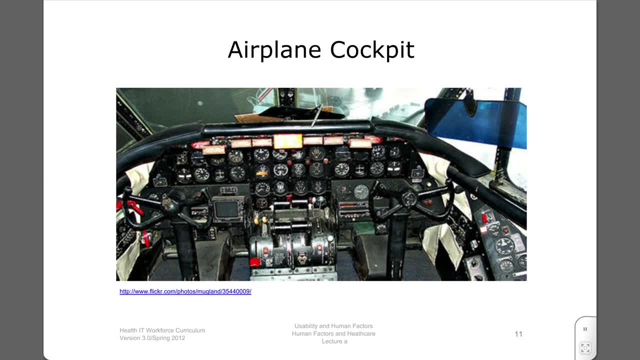 the healthcare sector has to some extent, patterned itself after the aviation industry. For example, checklists, structured communication techniques, air reporting and simulator training are some of the ways in which the healthcare sector has endeavored to adopt the safety and safety standards. 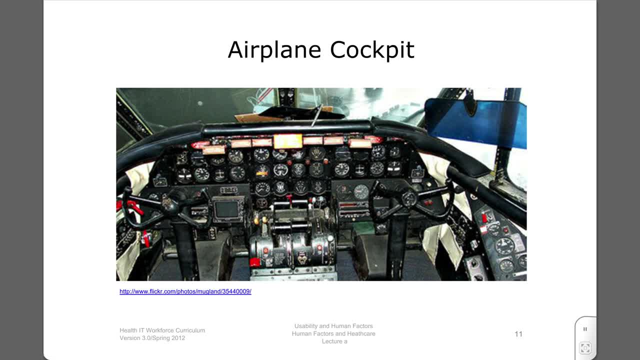 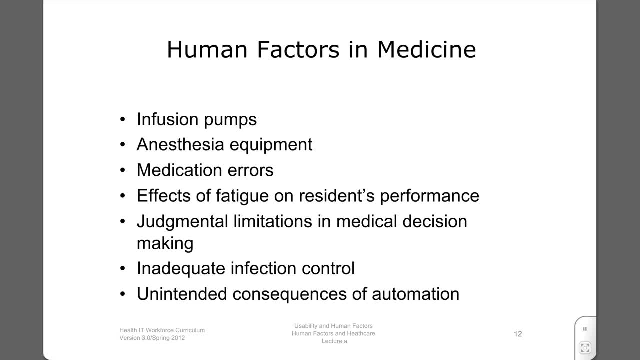 These are some examples of applications of human factors work in medicine. Infusion pumps are used to infuse fluid and medications into patients' circulatory system. In recent years, there have been growing concerns about the safety of these devices. Over one million patients are injured annually by medication errors. 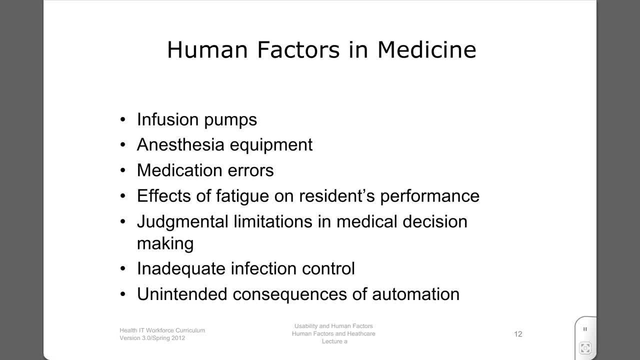 Although most are relatively minor, some result in serious patient harm and even fatalities. The effects of fatigue, night shift work and sleep deprivation on human performance and the safety of medical care are subjects of enormous interest within the medical community, Although this remains a controversial issue. 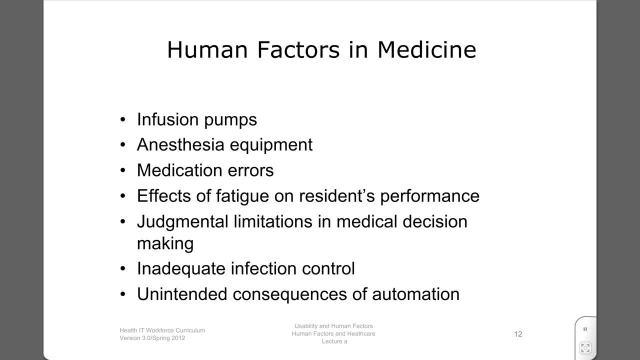 several states have mandated that medical residents limit the number of consecutive hours in a given shift. Infection control continues to be a serious problem in hospitals. Intervention like the close scrutiny of hand-washing behavior of clinicians has had a significant impact on controlling infection rates in hospitals. 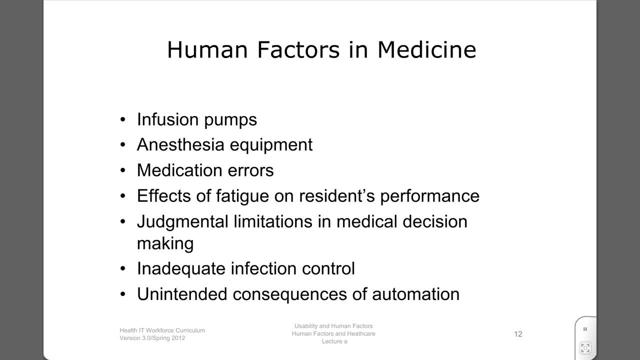 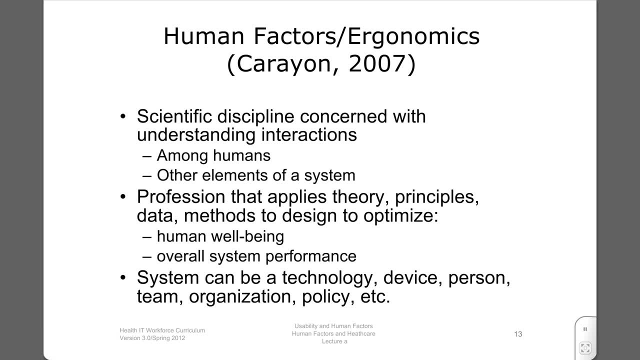 We will return to the issue of patient safety after we review some of the core concepts and central issues in human factors. As we discussed previously, human factors is a profession that applies theory, principles, data methods to design in order to optimize human work. human factors is a profession that applies theory, principles, data methods to design in order to optimize human work. human factors is a profession that applies theory, principles, data methods to design in order to optimize human work, human well-being and overall system performance. 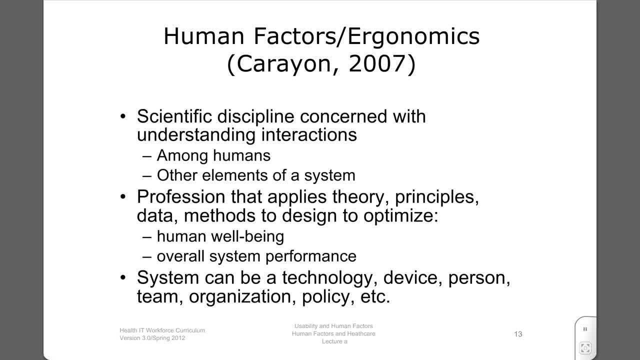 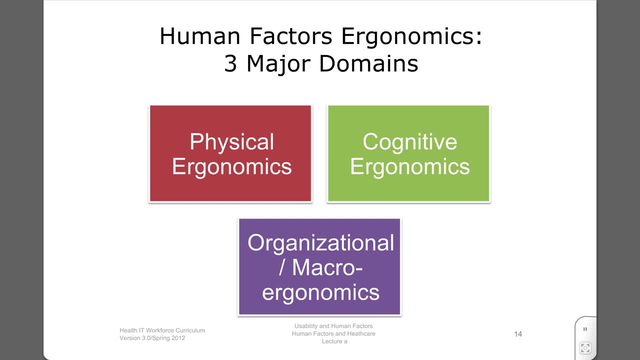 Unlike HCI, a system does not merely refer to a computing system. It may be a device, person, team, organization or policy, to name a few. Ergonomics is broadly conceived as the study of work and factors that affect it. 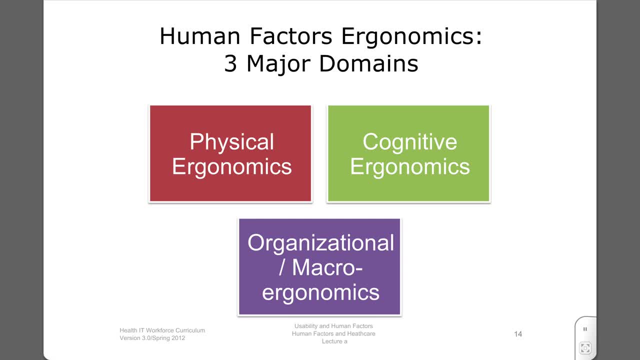 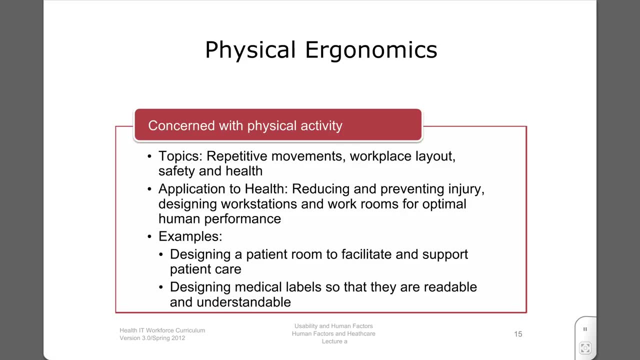 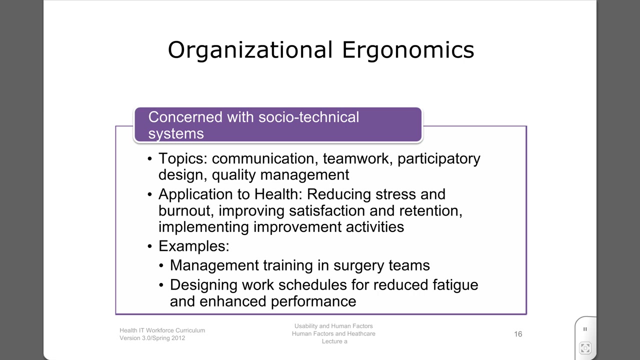 The term is sometimes used interchangeably with human factors. In any case, we can characterize three major domains. Physical ergonomics are concerned with physical activity and covers a wide range of related issues, including understanding and reducing injuries in the workplace. Organizational ergonomics is concerned with the study of socio-technical systems. 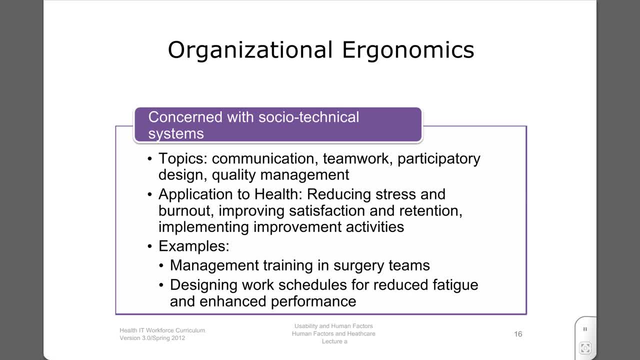 The topics in this area include communication, teamwork, participatory design and quality management. An example of an application to health is taking steps to reduce stress and employee burnout. Redesigning work schedules is one way to try and diminish the risk of burnout. 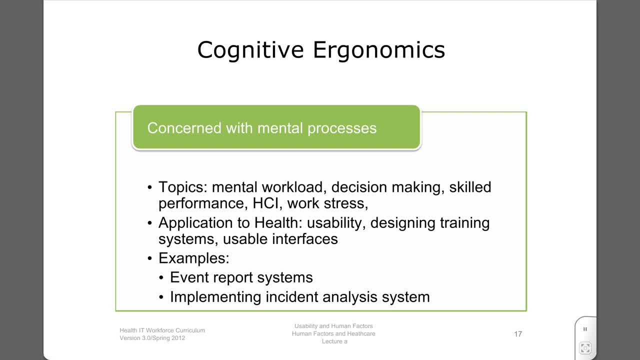 Cognitive ergonomics addresses the gamut of cognitive issues, including mental workload, an issue that we will come back to later in the presentation and usability of systems, which is a central issue in this course. This lecture focuses predominantly on cognitive issues. 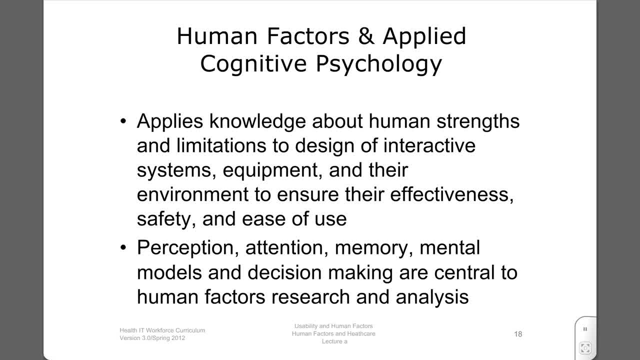 Human factors can be construed as a discipline guided by principles of engineering and applied cognitive psychology. Human factors analysis applies knowledge about the strengths and limitations of humans to design of interactive systems, equipment and their environments. The objective is to ensure their effectiveness, safety and ease of use. 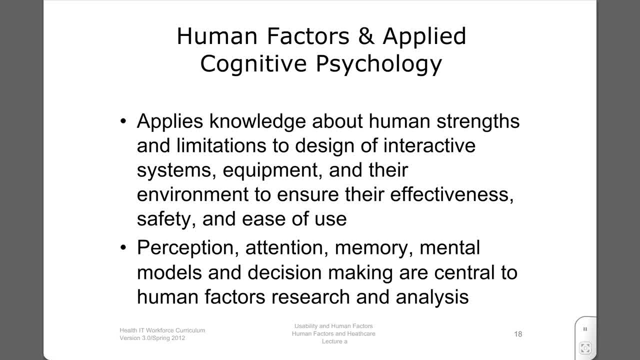 Mental models and issues of decision-making are central to human factors analysis. Any system will be easier and less burdensome to use to the extent that it is coextensive with users' mental models. We will now turn our attention to matters of attention. 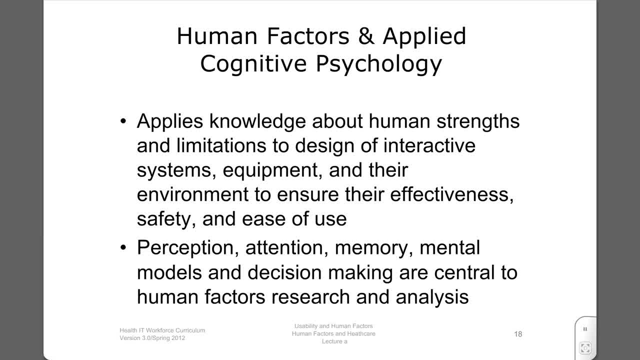 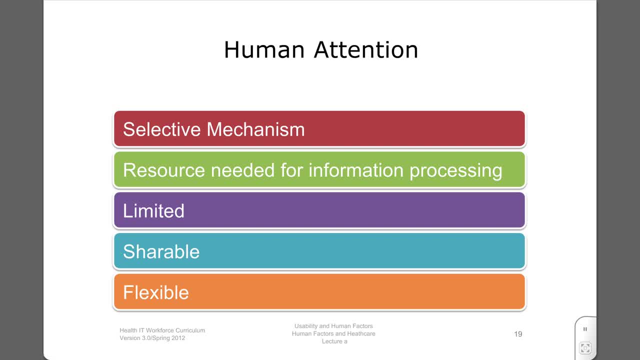 which is also a central concern in human factors analysis. Human factors focus on different dimensions of cognitive capacity, including memory, attention and workload. Our perceptual system inundates us with more stimuli than the cognitive system can possibly process. Attention mechanisms enable us to selectively prioritize. 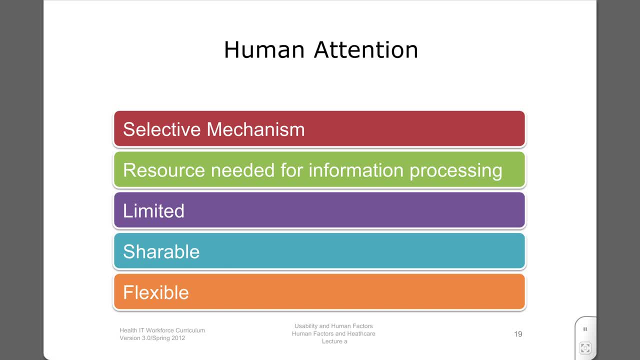 and attend to certain stimuli and attenuate other ones. Attentional resources are limited. They also have the proper use. They also have the property of being shareable, which enables us to multitask by dividing our attention between two activities. If we are driving on a highway, 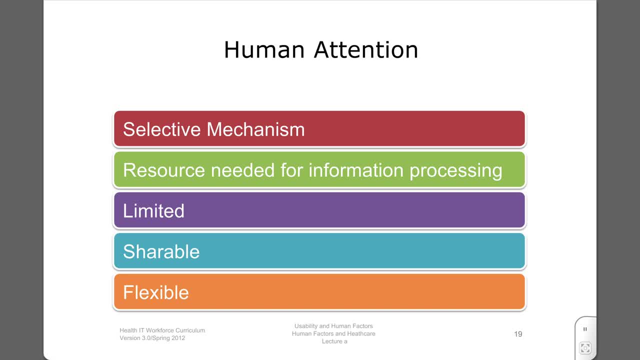 we can easily have a conversation with a passenger at the same time. However, as the skies get dark or the weather changes, or suddenly you find yourself driving through winding, mountainous roads, you will have to allocate more of your attentional resources to driving. 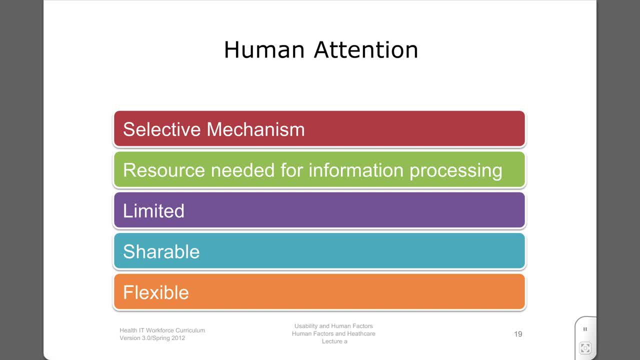 and less to the conversation. Most states have outlawed the use of hand-held cell phones while driving because they serve to divide one's attentional resources and greatly increase the likelihood of accidents and highway fatalities. On the basis of studies thus far, it is not clear that using a hands-free cell phone 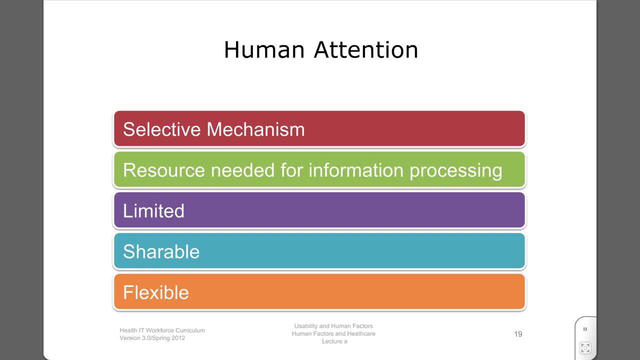 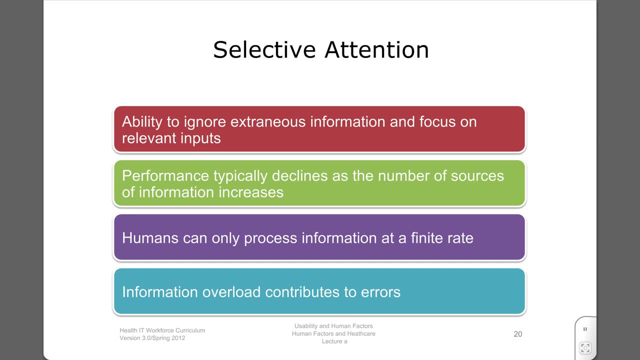 has any effect on reducing driving accidents. It has the effect of sapping one's needed attentional resources. We have the ability to ignore extraneous information and focus on relevant information. However, performance typically declines as the number of sources of information increases. 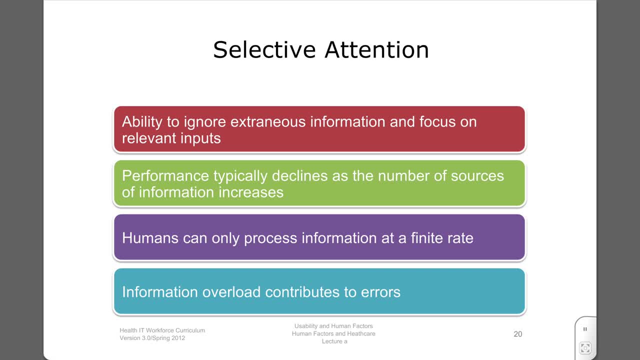 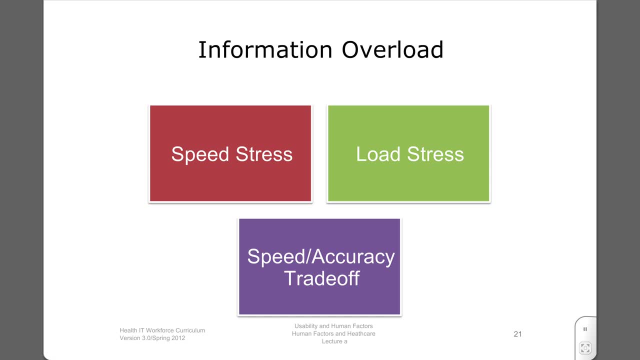 Information overload is a common cause of performance errors. This slide describes some of the conditions for overload. If you are under pressure to increase the pace of your performance or if you are burdened by heavy information load, the quality or accuracy of performance is likely to degrade. 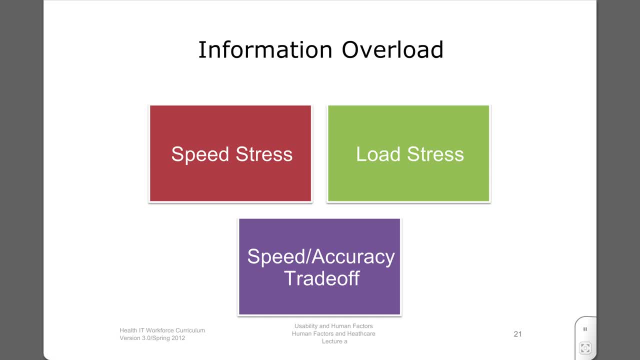 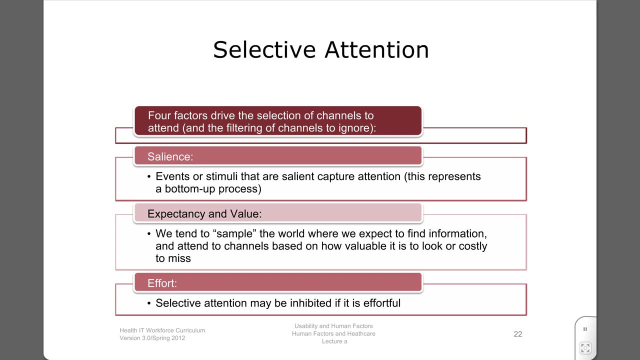 There is a speed-accuracy trade-off: As you increase your speed of performance beyond a certain threshold, you increase the probability that the quality or accuracy of your work will degrade. This slide enumerates a number of factors that drive the selection of channels to attend. 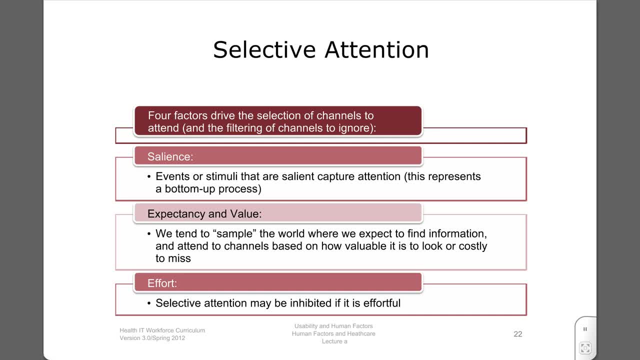 Events or stimuli that cause problems or events that are salient tend to capture our attention. Loud music or a conversation where someone mentions your name is likely to capture your attention. We tend to sample the world where we expect to find information and attend to channels based on how valuable it is to look. 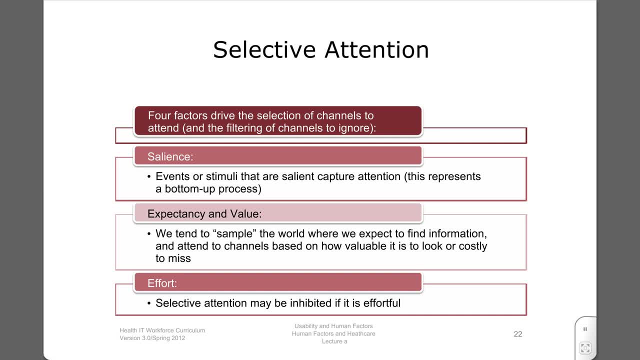 or costly to miss. This can be a property of expertise. Nuclear power plant operators or intensive care nurses are trained to attend to particular signals that are vitally important. If we are inundated with stimuli, such efforts may be fruitless. For example, 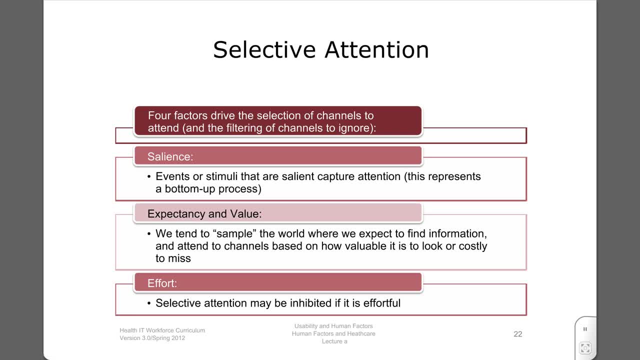 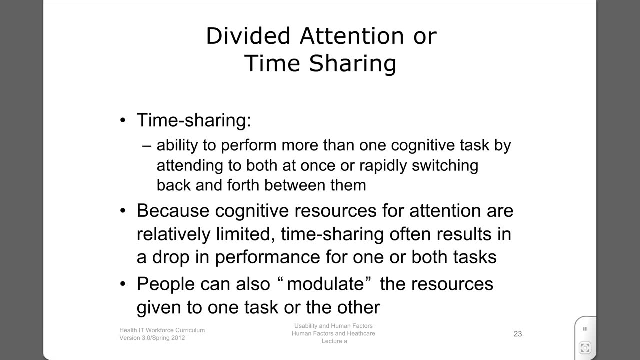 trying to study complex subject materials in a noisy café may be very effortful. On the other hand, we may be able to read a newspaper or a novel in the same environment. Time sharing refers to the ability to perform more than one cognitive task by attending to both at once. 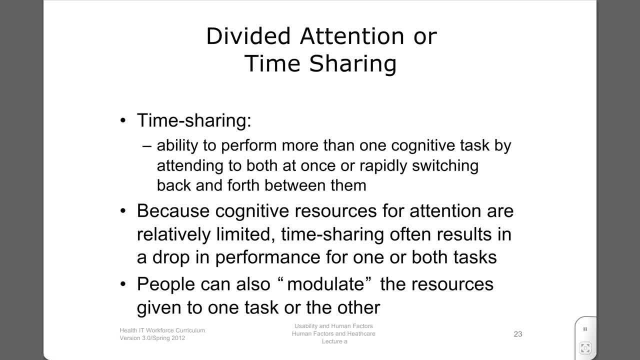 or rapidly switching back and forth between them. We routinely divide our attention when working on our computer, We may be writing, listening to music and watching out for an important email. However, given the fact that cognitive resources for attention are relatively limited, 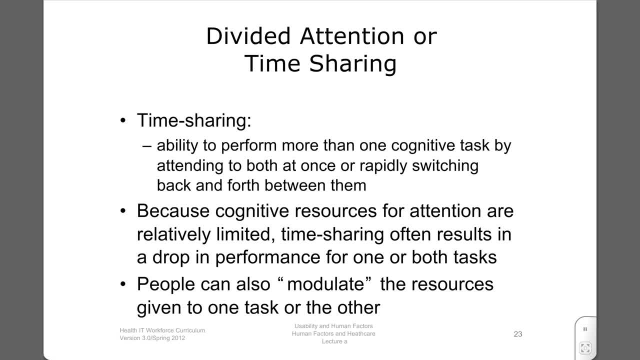 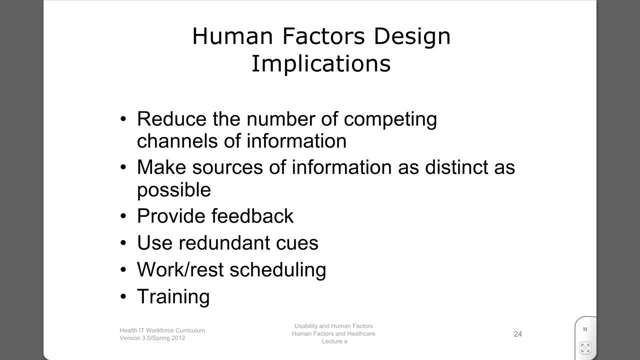 time sharing often results in a drop in performance for one or both tasks. We can modulate our attention resources by giving more attention to the task that is more important at the moment. On the basis of human factors research, we can draw the following design implications: 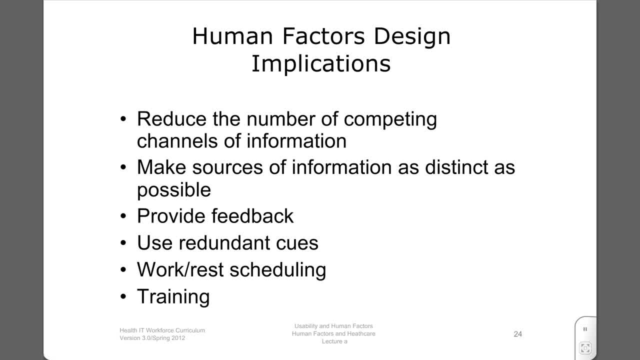 If possible, reduce the number of channels that one needs to attend to Make sources of information as distinct as possible. For example, an intensive care nurse may hear 10 or 12 different kinds of alarms that signal various kinds of patient needs or concerns. 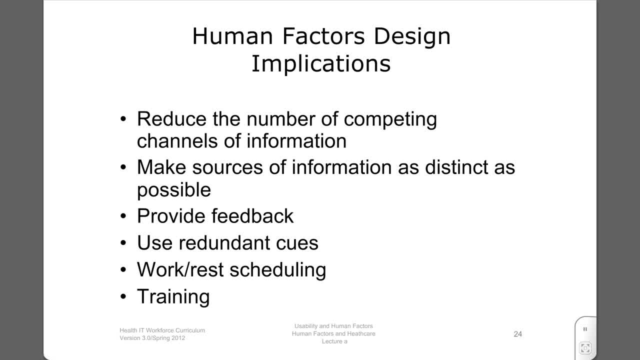 However, the sounds are sufficiently distinct that he or she will know which ones warrant immediate attention and which ones can wait a little longer. Electronic health records can be designed or templates developed that correspond better to the desired clinician workflow, and displays can be structured. 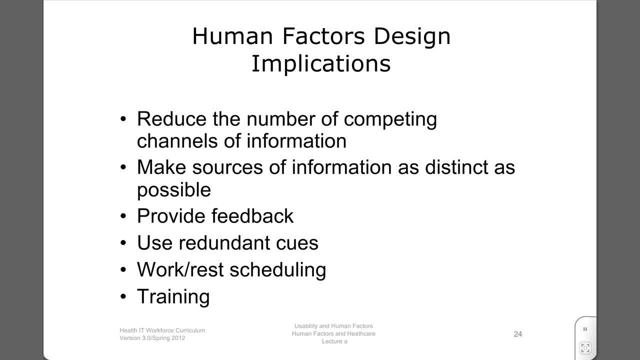 to provide easier access to needed information. Work scheduling can be used to reduce fatigue and improve performance. Although training is not a substantive task, training is not a substitute for poor design. it can provide workers with strategies and resources to work more productively within the limitations of a given system.